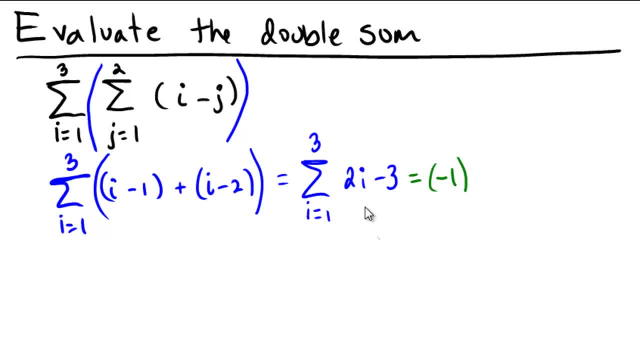 Then we would replace i for 2,. 2 times 2 is 4,. 4 minus 3 is positive 1.. And then we replace i with 3, right, which would now be: 2 times 3 is 6, minus 3 is 3,. 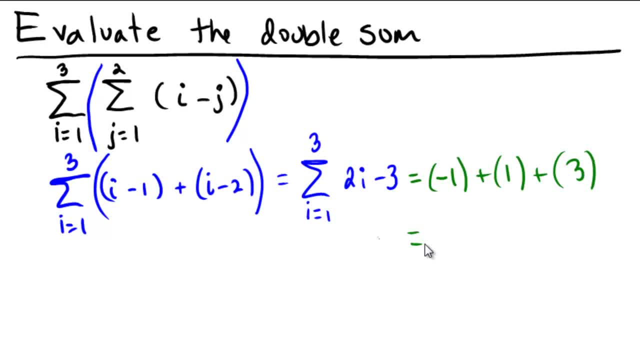 and then we would add those together: Minus 1, plus 1 is 0,, plus 3 is 3, and so that's So. our final answer to this double sum is positive 3.. So now, why don't you pause the video and see if you can do this one on your own? 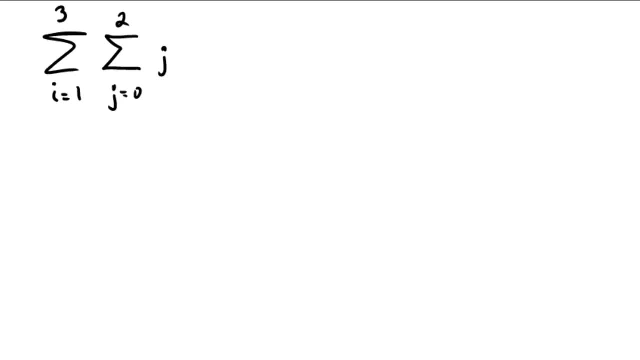 The sum i equals 1 to 3 of the sum j equals 0 to 2 of just j. So there is no i floating around this time. So, assuming you paused the video and gave this a good old shot here, let's see what we can do together. 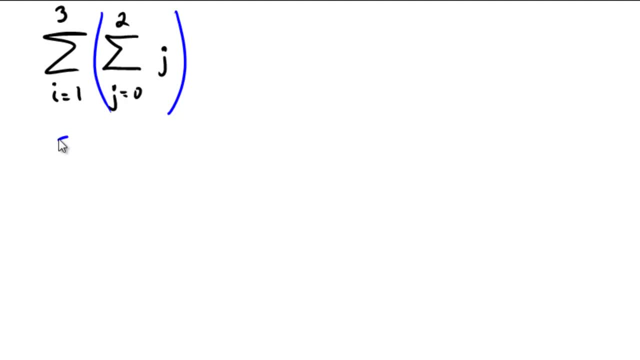 I'm going to put some parentheses around that so that we're doing the sum i equals 1 to 3, of now I'm going to replace j equals 0 to 2 in each increment of the index. So if we replace j with 0,, we get 0.. 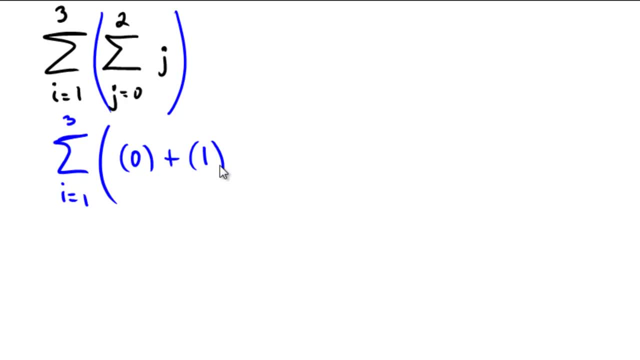 If we replace j with 1,, we get 1, and if we replace j with 2,, we get 2.. So inside of there we have 0 plus 1 plus 2.. So this is going to be equal to the sum i equals 1 to 3,. and 0 plus 1 plus 2.. So this is going to be equal to the sum. i equals 1 to 3, and 0 plus 1 plus 2.. So 0 plus 1 plus 2 is just the number 3.. 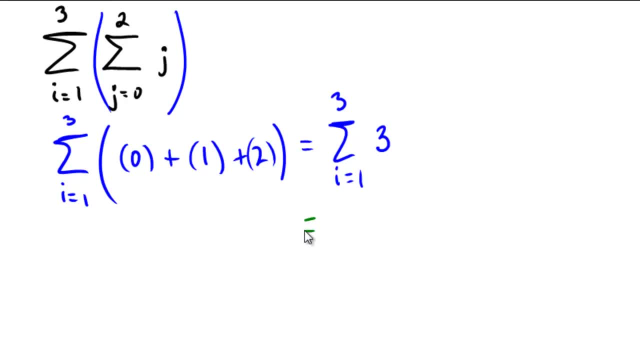 So now we're ready to do the summation on the i index. So if I were to replace i with 1,, what do we get out of this argument? Well, it looks like we just get a 3, because there is no i. 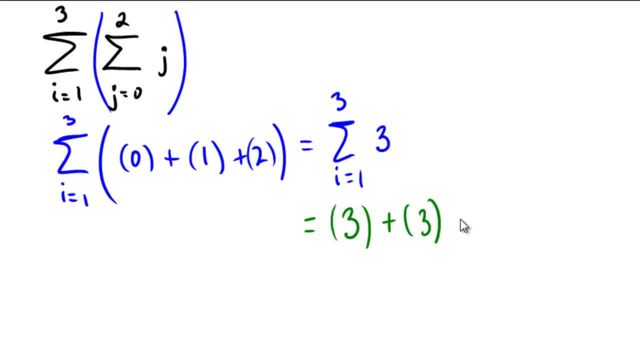 If we replace i with 2, we also get 3, and if we replace i with 3, we just get 3.. Right, because there's no i in the argument, so we just get whatever the output says, and that's 3.. 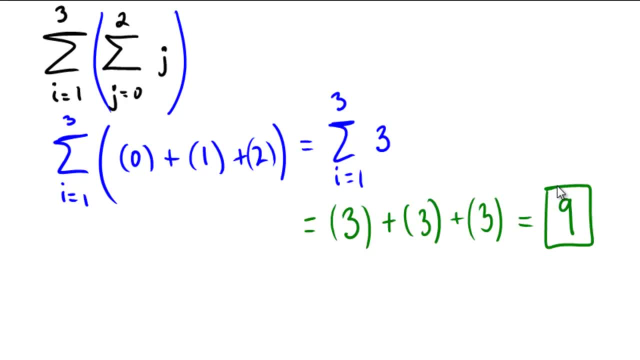 3 plus 3 plus 3,, of course, would be 9,, and that's the final answer for this double sum. 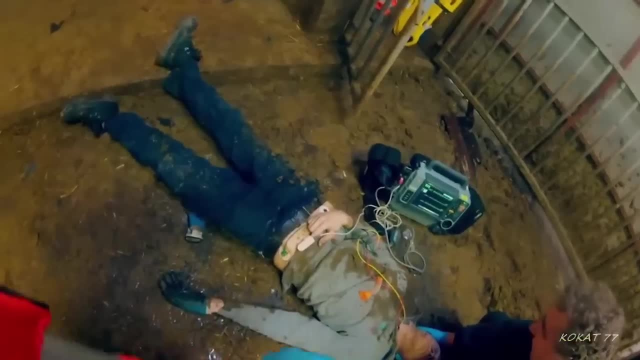 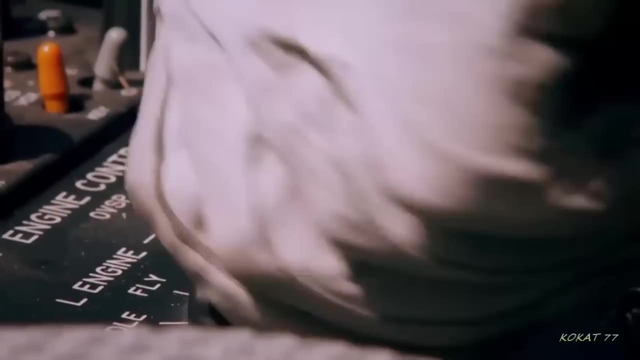 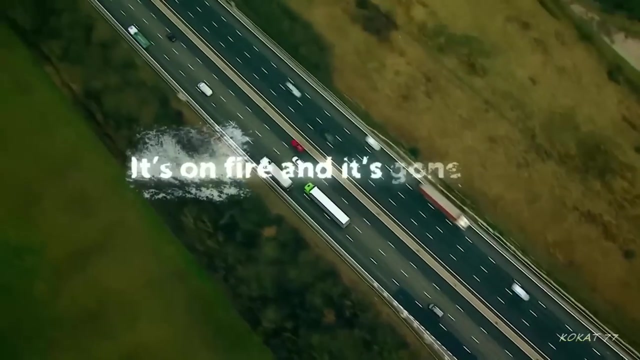 Breathing. He's struggling to breathe, Very seriously injured In some of the UK's most remote places. Stay on the line and I'll tell you exactly what to do next. There's just been an accident on the M1 motorway. He's on fire and he's gone into the railway bridge. Your